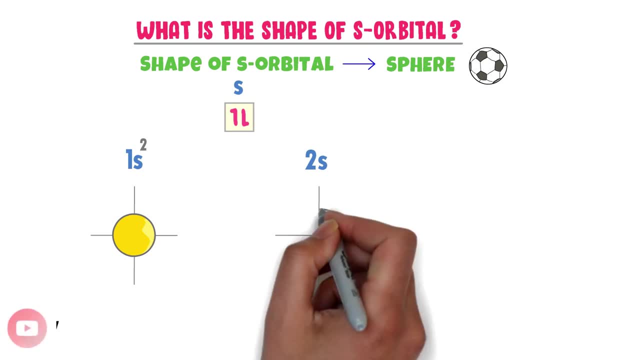 region. Now consider 2s. The ship of 2s is also spherical, but its size is bigger than 1s. We know that 2s can also accommodate two electrons. Thus you can find the two electrons of 2s in this spherical. 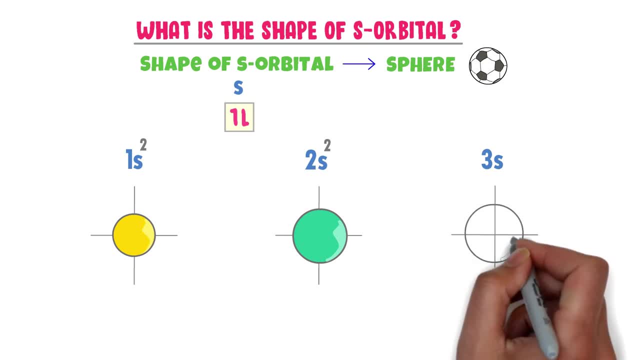 region. Consider 3s. The ship of 3s is also spherical and its size is bigger than 2s. Thus you can find the two electrons of 3s in this spherical region around the nucleus. Just remember that the shape of S-orbital is sphere like a ball. 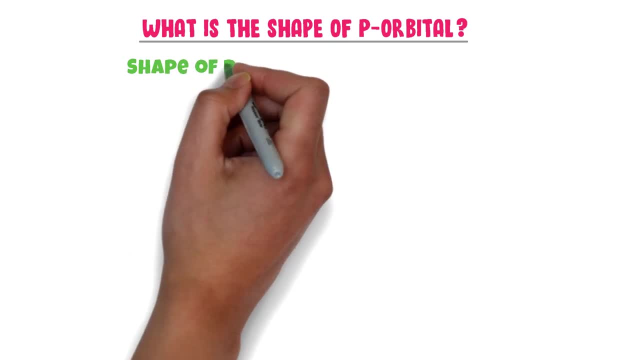 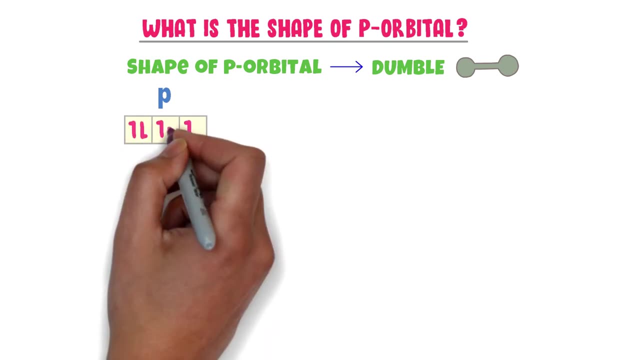 Now, what is the shape of P-orbital? Well, the shape of P-orbital is like a dumbbell. We know that P-orbital can accommodate 6 electrons. P-orbital has three degenerate orbital: 2px. 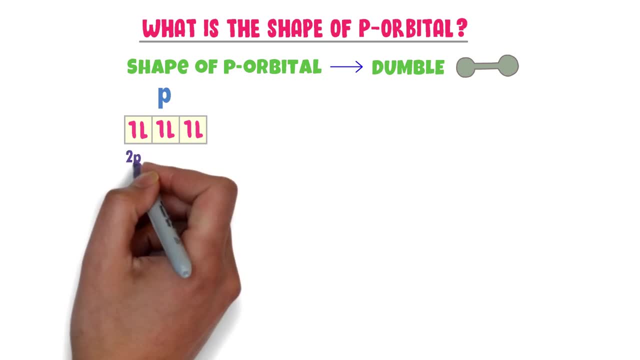 2py and 2pz. You will learn in this lecture that why we call these orbitals 2px and 2px, and then why we call these orbitals 2px and 2pz. Yes, Yes, Yes. 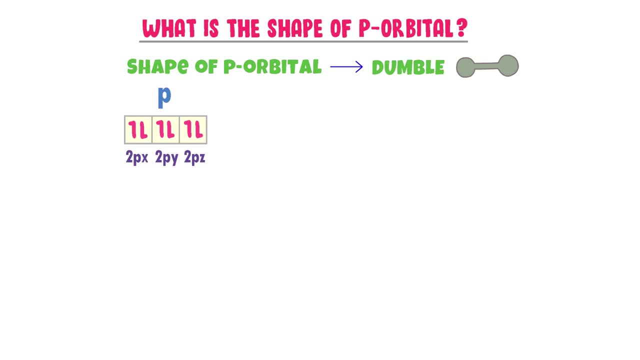 2py and 2pz. Now each orbital of p can accommodate two electrons. Here let me draw the shapes of 2px. Draw the two axes, x-axis and y-axis. 2px means that draw the p orbital along the x-axis. So I 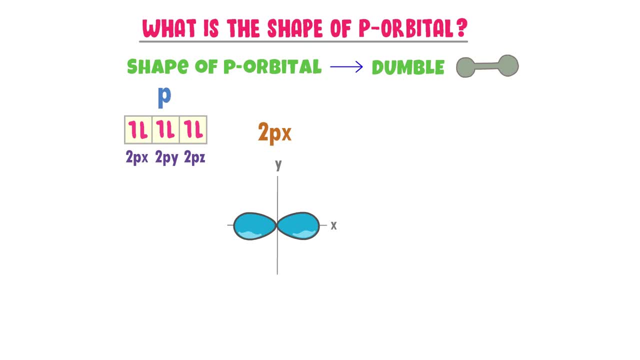 draw dumbbell shape along the x-axis. We know that 2px can accommodate only two electrons. Thus in 2px orbital you can find the two electrons along x-axis in this region. Secondly, let me draw the shape of 2py Again. draw the two axes, x-axis and y-axis. 2py means that draw the p orbital. 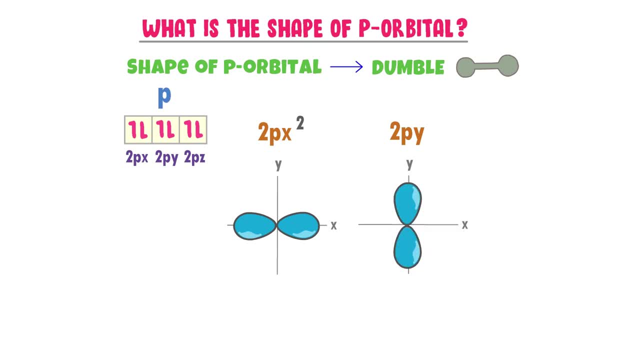 along the y-axis. We know that 2py can also accommodate two electrons. Thus in 2py orbital you can find the two electrons along the y-axis. So I draw dumbbell shape along the y-axis. 3. Let me draw the shape of 2pz. Now draw the three axes: x-axis, y-axis and z-axis. 2pz means that 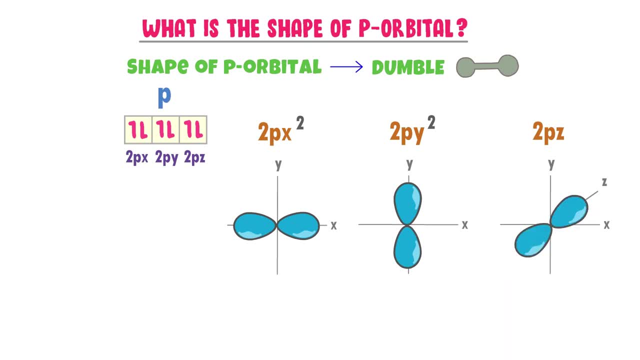 draw the z orbital along z-axis. We know that 2pz can also accommodate two electrons. Thus in 2pz orbital you can find the two electrons along z-axis in this region. Hence note it down that 2p orbital oriented along x-axis is called 2px. 2p orbital oriented along y-axis is called 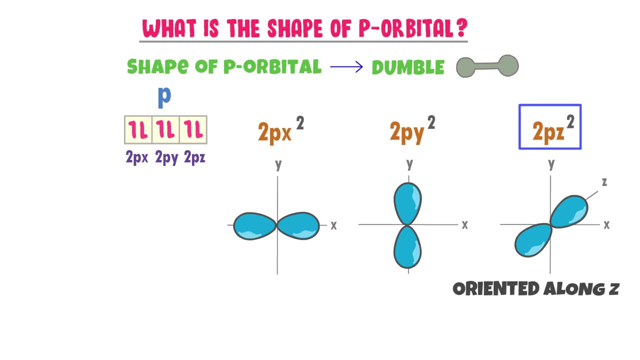 2py and 2p. orbital oriented along z-axis is called 2pz. Here is a bonus tip for you: 2px, 2py and 2pz are orthogonal. It means that 2px is perpendicular to 2py and 2py is perpendicular. 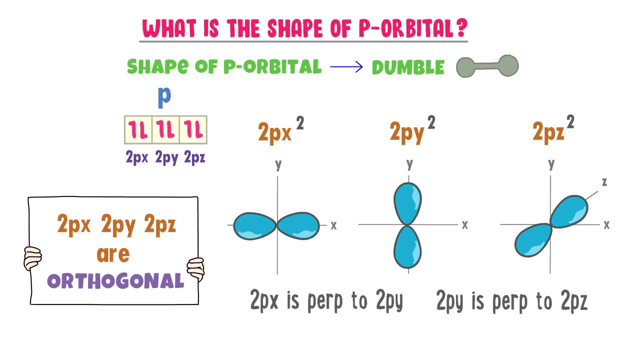 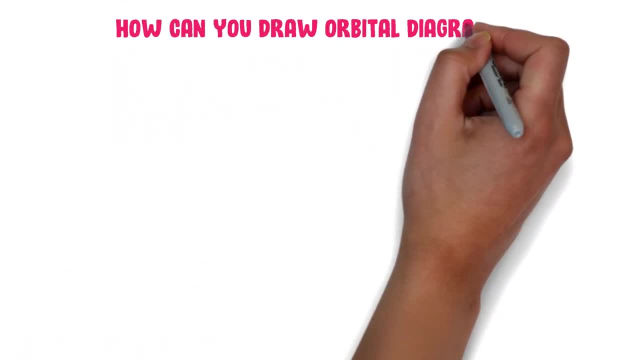 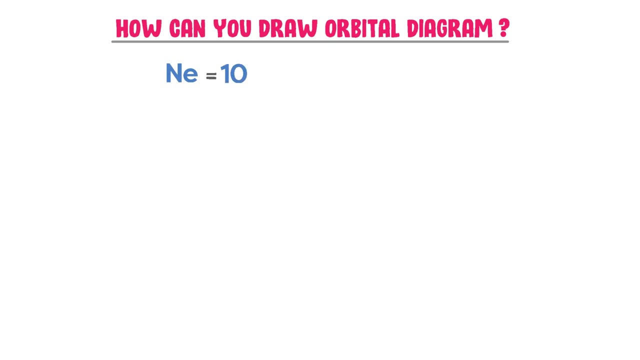 to 2pz. So they all are perpendicular to each other. Hence they all are orthogonal. Now how can you draw orbital diagram and electronic configuration of atom like neon? The atomic number of neon is 10.. 1s can accommodate two electrons. 2s can also accommodate two. 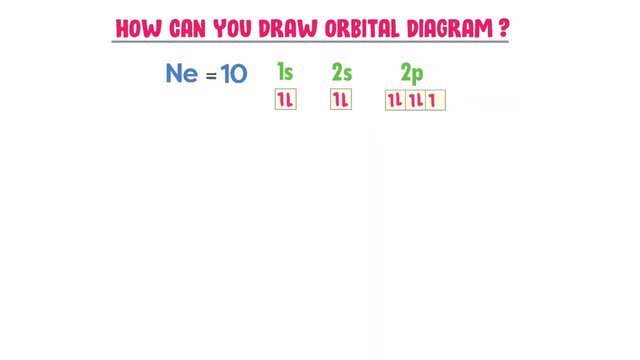 electrons, and 2p can accommodate six electrons and 2px, 2py and 2pz. Hence I configure the ten electrons of neon. Now I draw two axes: x-axis and y-axis. I intentionally do not draw z-axis, because I want things to be neat and clean. Firstly, I draw 1s orbital. 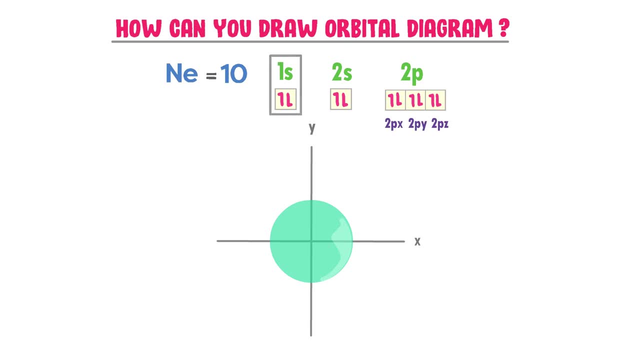 and the two electrons of 1s are present in this region. Secondly, I draw 2s orbital and the two electrons of 2s are present in this region. Then I draw the 2px orbital along x-axis, Then I draw the 2py orbital along y-axis and 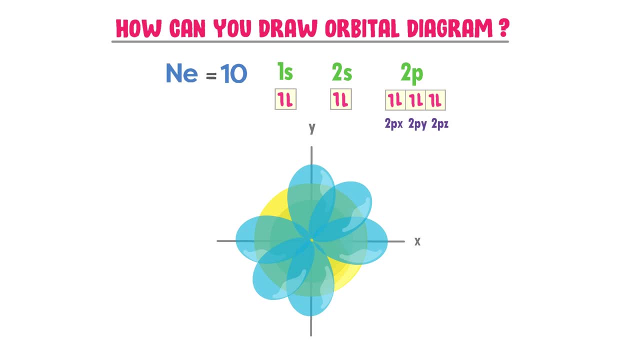 I draw 2pz orbital along z-axis. Thus, this is the orbital diagram and electronic configuration of neon atom. By this way, you can draw the atomic orbitals of any atom. Finally, what is the shape of d-orbitals? Well, the shape of d-orbitals is like double-double. 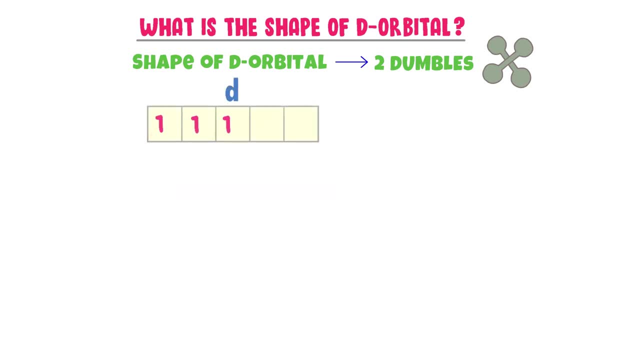 We know that d-orbital can accommodate 10 electrons. So it has five degenerate orbitals And each orbital can accommodate only two electrons. Now how to name these degenerate d-orbitals Here? let me teach you my personal trick. I write xyz at one side of the page. 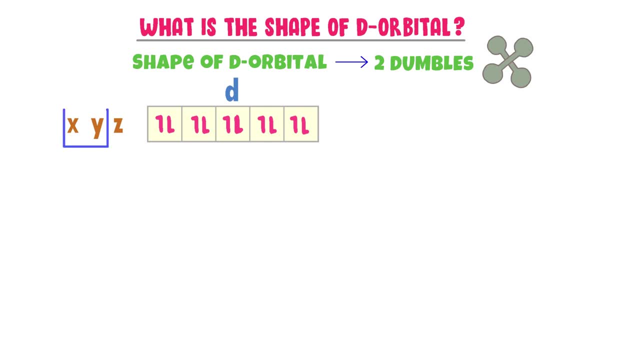 and go from x to z. Firstly I take xy and write here as z, Then I write z as z And finally I write z as z. So I draw the z-orbitals, I write z as z, I draw the z-orbitals, I draw. 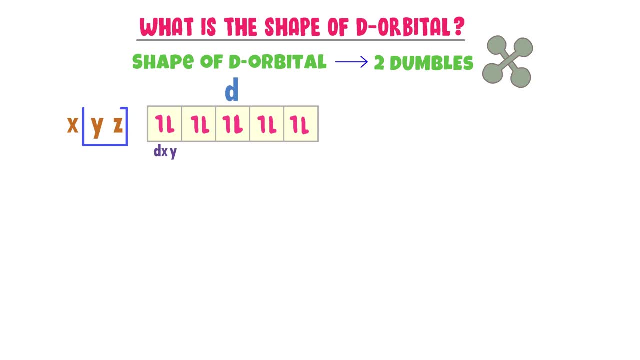 the z-orbitals. I draw z as z, I draw z as z And finally, I draw z as z. I draw z as z. I draw as dxy. then I take yz and write it here as dyz. then I take xz and write it here as dxz. 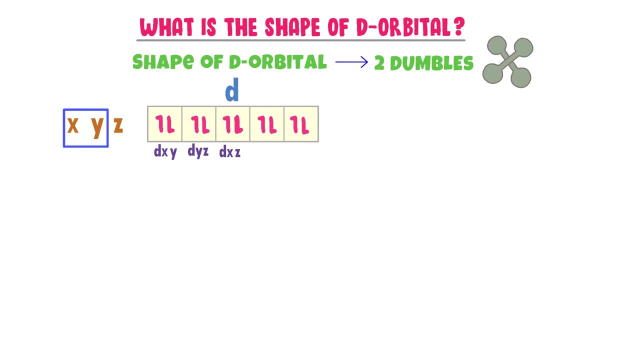 now I take x squared minus y squared and write it here as dx squared minus y squared. and lastly, only z is remaining, so I write it as dz squared. Now, if I draw the three dimensional shape of d orbitals, it is difficult and time consuming. 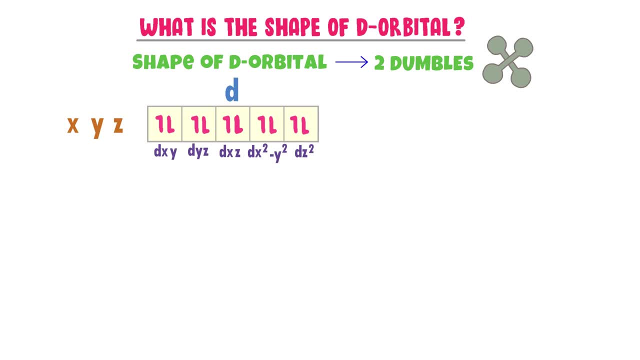 an exam. hence I will teach you the two dimensional shapes of d orbitals, but you must also understand the system of three axes. These three axes are orthogonal. it means that these three axes are perpendicular to each other. I will select only two axes in order to draw the neat and clean shapes of d orbitals. 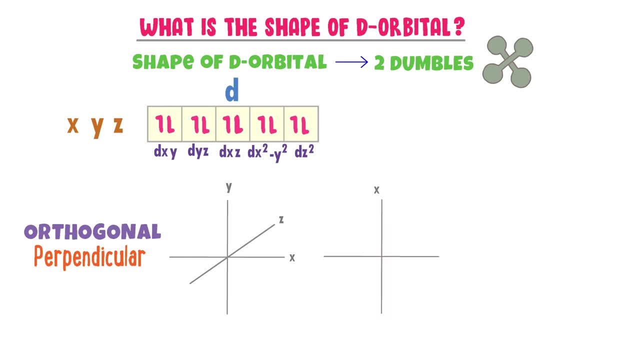 For example, I can take x axis in this direction and y axis in this direction, but they must be perpendicular. Similarly, I can take z axis in this direction and y axis in this direction. Now let me take dxy orbital. I will only draw the x axis and y axis. 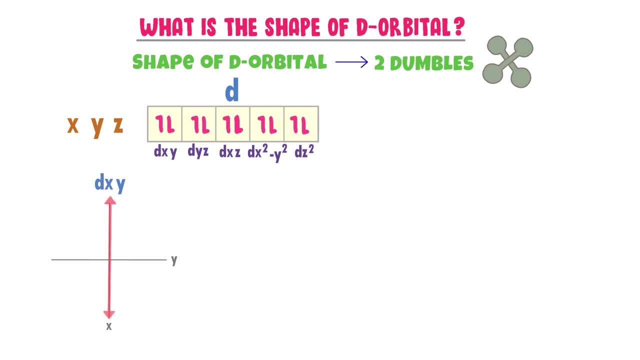 Remember that you can take y axis in this direction and x axis in this direction, but it must be perpendicular, So it all depends upon you. dxy means that the d orbital is present in between x axis and y axis, and we also know that the shape of d orbital is like double dumbbell. 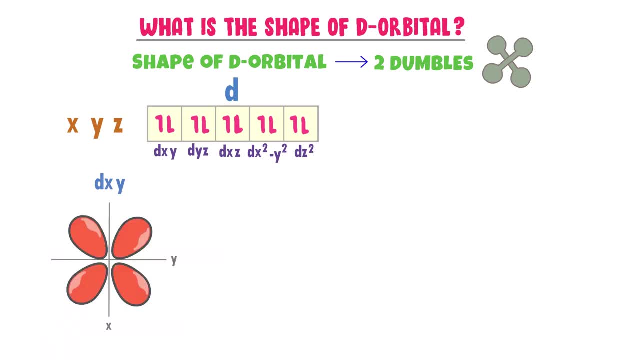 So I draw the double dumbbell shape in between x axis and y axis. So in dxy orbital you can find the two electrons in between the x axis and y axis in this double dumbbell region. Now let me take the dy shape. 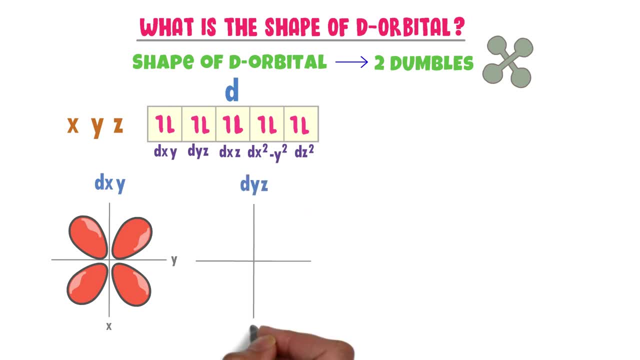 At that time I will take dxz. Secondly, I draw y axis in this direction and z axis in this direction. I draw the double dumbbell like shape in between them. So in dyz you can find the two electrons in between y axis and z axis. 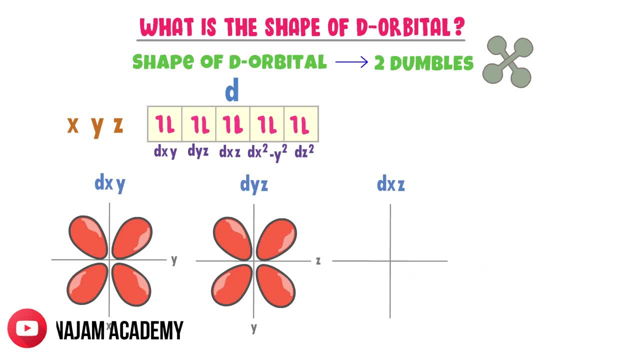 Thirdly, I take dxz. I draw z axis in this direction and x axis in this direction. Now I draw the double dumbbell like shape in between the two x's axis. So in dxz you can find the two electrons in between this region. Fourthly, I take the dx. 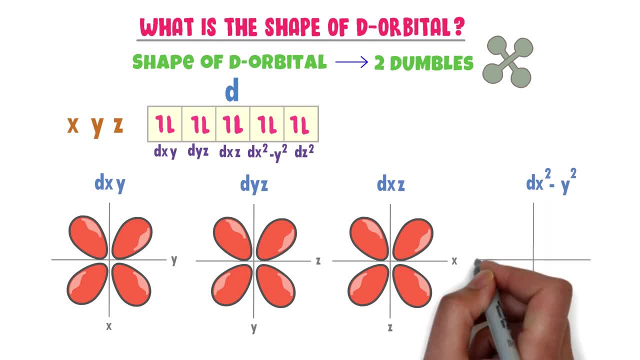 squared minus y squared, I draw the x-axis in this direction and y-axis in this direction. Here is my personal trick to draw the shape of dx squared minus y squared. This minus sign between them means to draw the d-orbital along x-axis and y-axis. So I draw the d-orbital along x-axis. 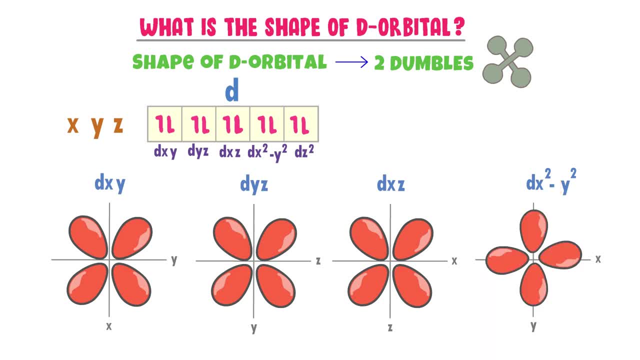 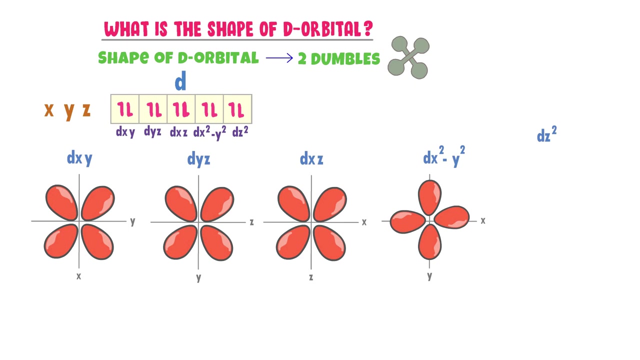 and y-axis and I get dx squared minus y squared orbital. Remember that in case of dx squared minus y squared orbital, you can find the two electrons along x-axis and y-axis. Lastly, let me take the dz squared orbital. Here a lot of students are confused. They are confused about drawing z-axis and x-axis or z-axis. 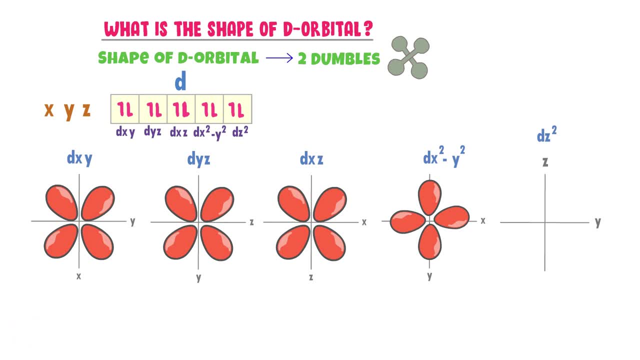 and y-axis. Well, you can draw either of these two systems. Both are correct. The shape of dz squared is like a single dumbbell, but draw it along z-axis and the donut-like ring at the center of x-axis Also. remember that. 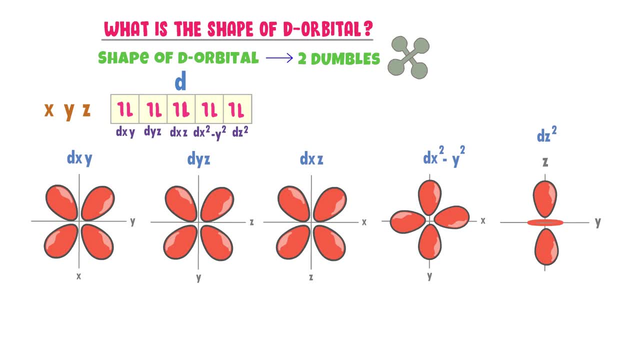 you can draw the d-orbital along x-axis and y-axis, You can find the two electrons of dz squared along z-axis. Thus, these are the five shapes of d-orbitals. I hope that you have learned all about the shapes of orbitals.